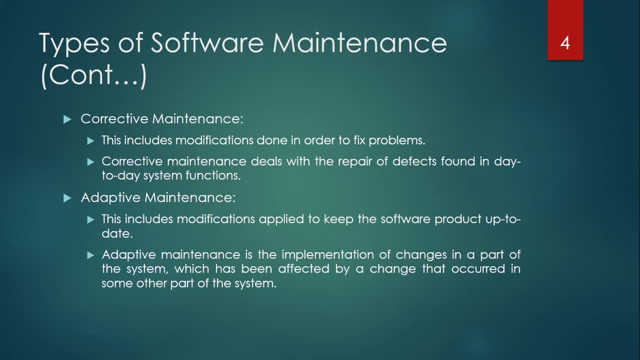 Second one is adaptive maintenance. Adaptive maintenance includes modification applied to keep the software product up to date. Adaptive maintenance is the implementation of changes in a part of the system which has been affected by a change that occurred into some other part of the system. If we have updated our software, if we have updated any part of our software so that updation can affect to the other operation, other systems. 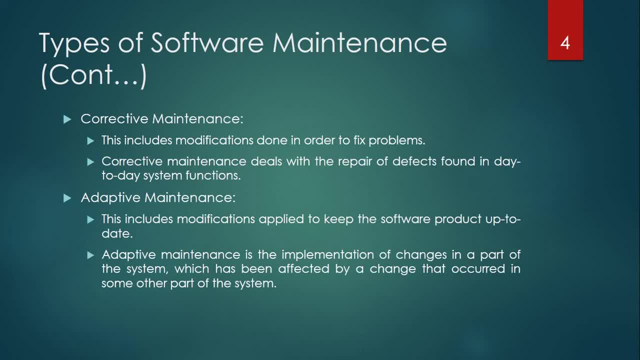 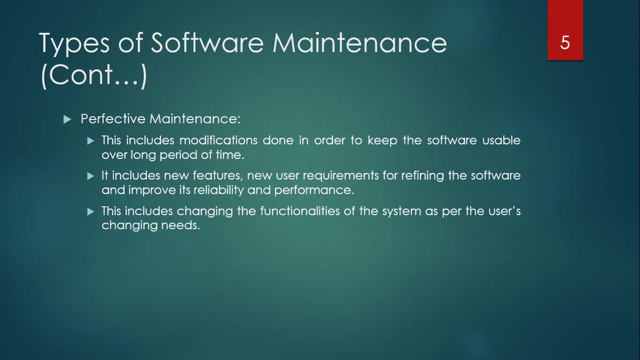 So we will have to maintain that other system, that other operation also. So that type of maintenance will be known as adaptive maintenance. Adaptive means with update. if affected any part, then we will have to maintain that part. That means adaptive maintenance. Third maintenance is perfective maintenance. 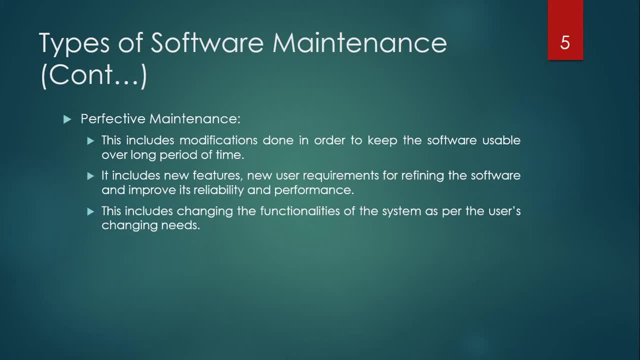 This includes modification done in order to keep the software usable over long period of time. It includes new features, new user requirement for refining the software and improve its reliability and performance. This includes changing the functionality of the system as per the user changing need. 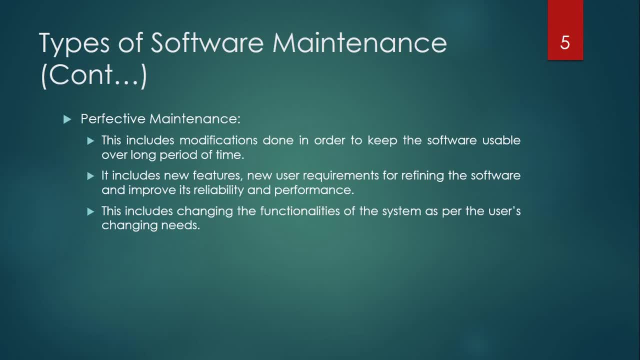 Perfective maintenance means if we have developed a software, that software is used by the user. After some time user needs some more features into that software, So that type of maintenance will be known as the perfective maintenance. We will make our software more perfect then. that is the perfective maintenance. 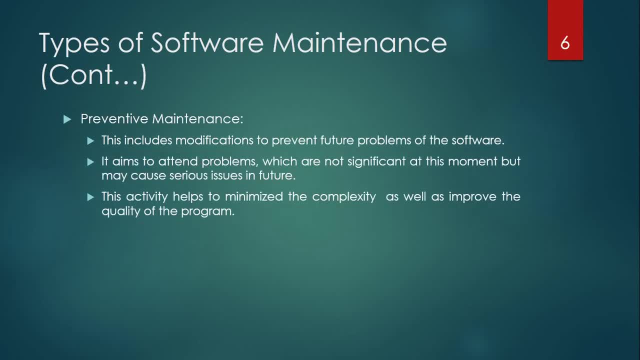 Last is preventive maintenance. This includes modifications to prevent future problem of the software. It aims to attend problem which are not significant at this moment but may cause serious issue in the future. This activity helps to minimize the complexity as well as improve the quality of the program.